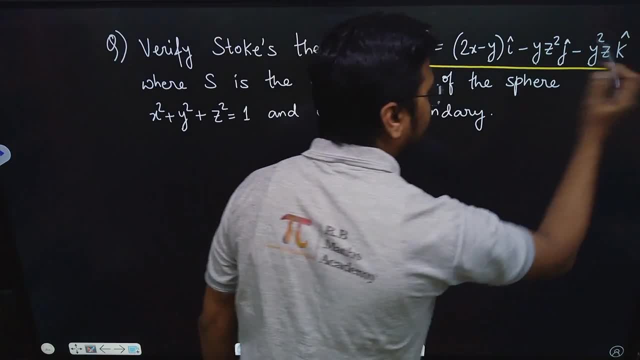 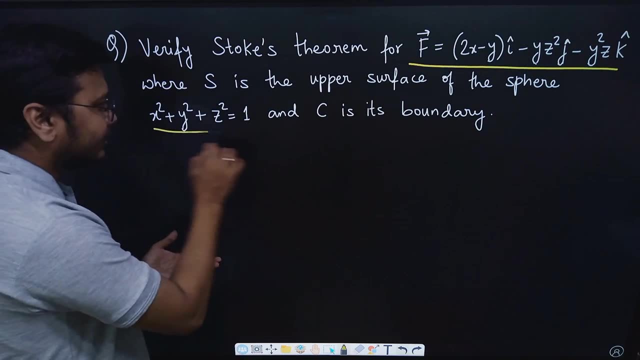 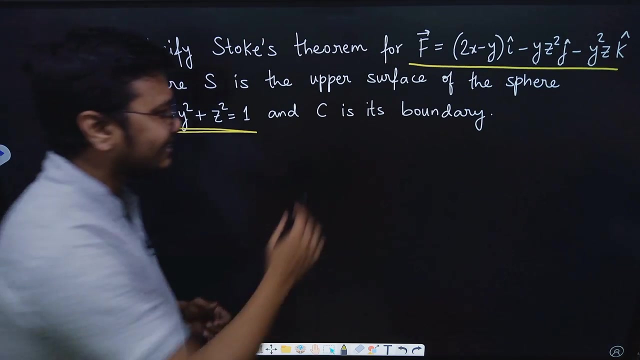 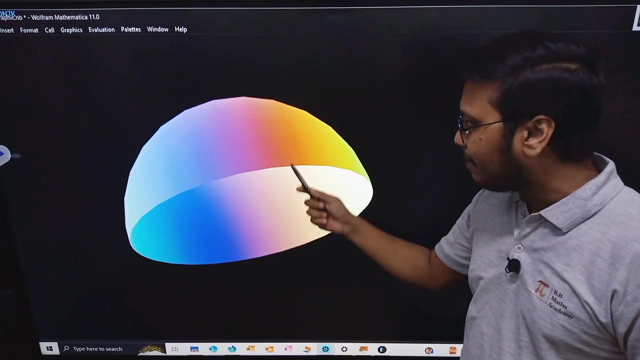 we need to verify Stokes theorem for this particular given function- vector function. where s is the upper surface of the sphere? where the sphere is given by something like this, That means upper surface of the sphere, means we are dealing with a hemisphere, Okay, and c is basically the boundary of that hemisphere. So let's take a look at the hemisphere. So this is the hemisphere that we have. You can see, this is the upper part of the hemisphere, and 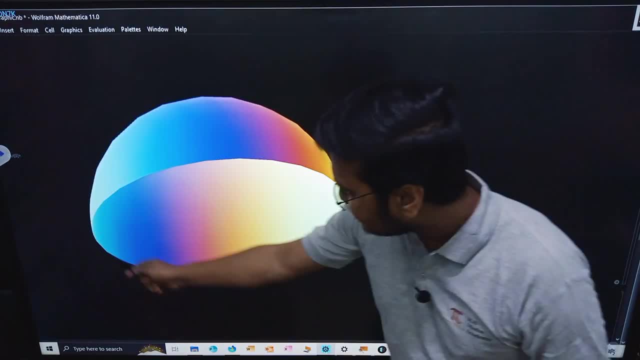 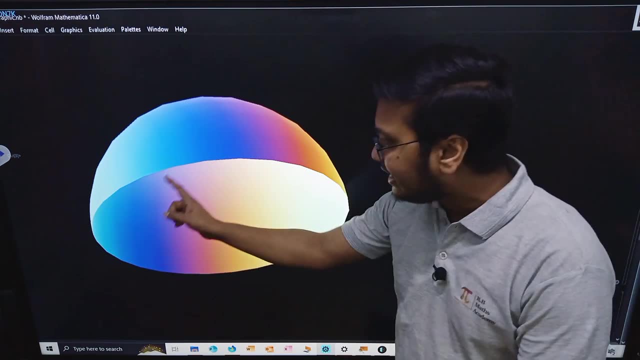 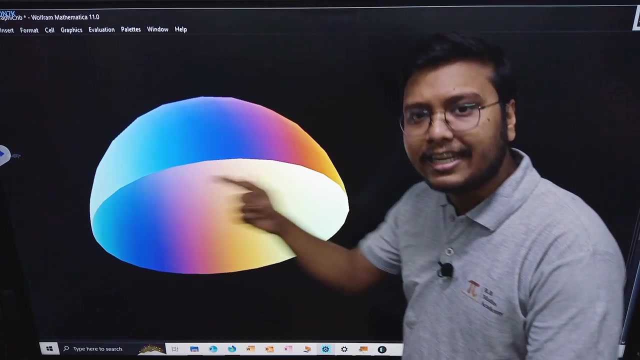 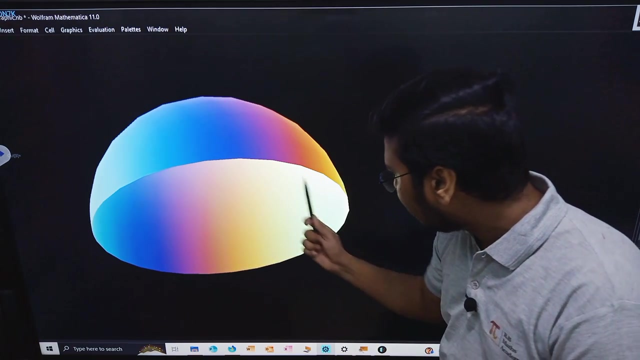 this is the boundary. As you can see, this is the boundary of the hemisphere. That means this is the c boundary. This boundary is represented by c and we have to take the c boundary in a sense that if a right handed screw would rotate in that direction, in the direction in which it would advance, that would be the direction of n cap. So you can assume that here the direction must be something like this, The way I am moving my hand. 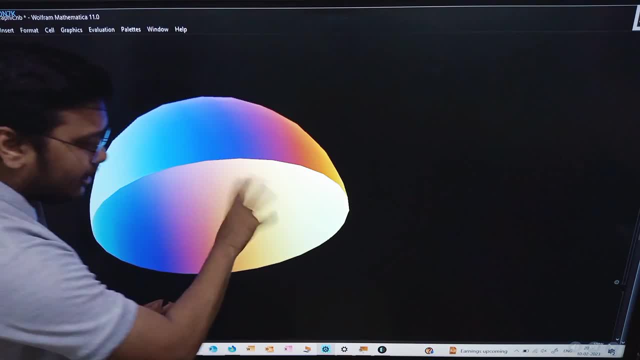 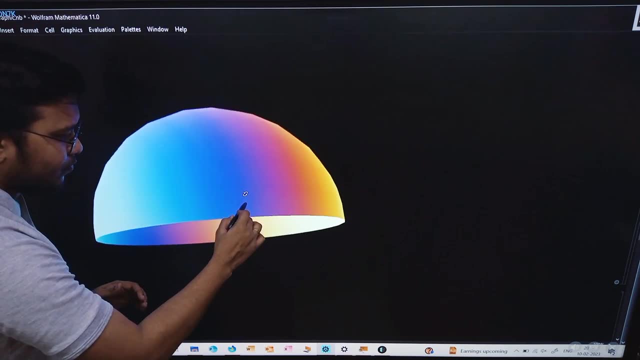 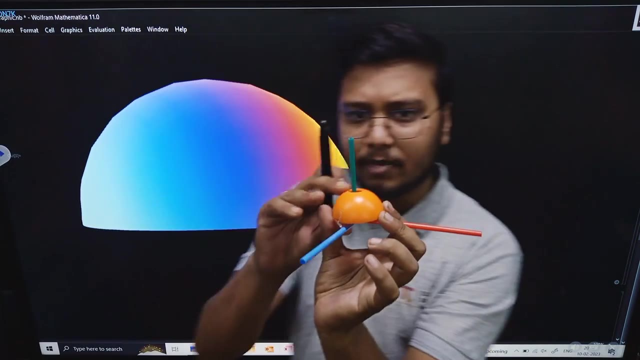 If I move it in this manner, then the right-handed screw that would advance inside the blackboard. So that means, if I just assume that if I keep my hemisphere in this way so you can compare, that this is basically the hemisphere that I have over here in my hand and you can see. 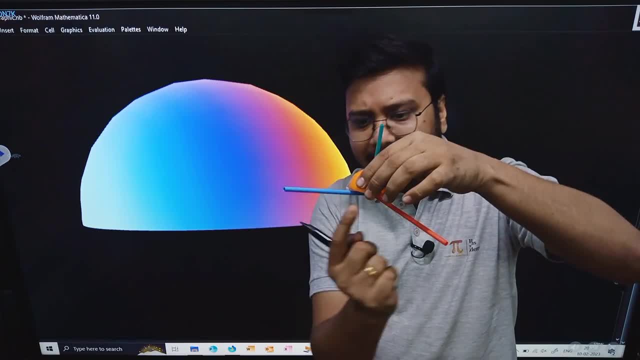 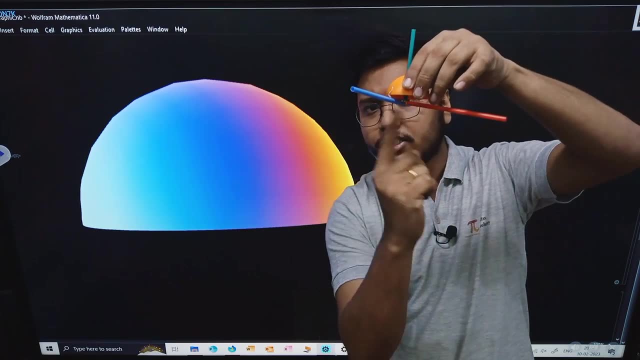 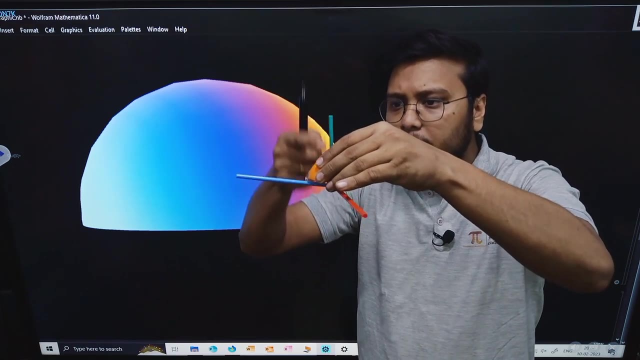 on the board. So if I take it in a way that the C curve, we are moving along the C curve in this particular direction, if you follow my finger in this particular direction, then it would advance in the direction of this green line, which I can assume is the Z axis. 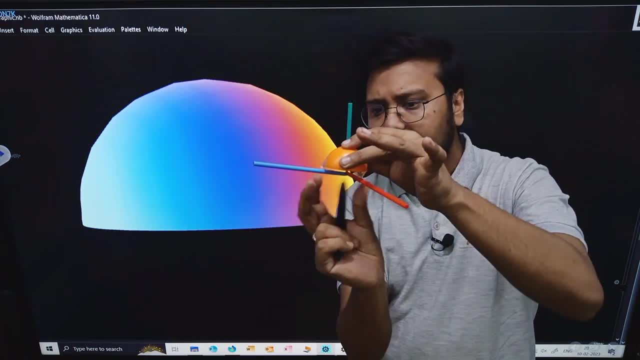 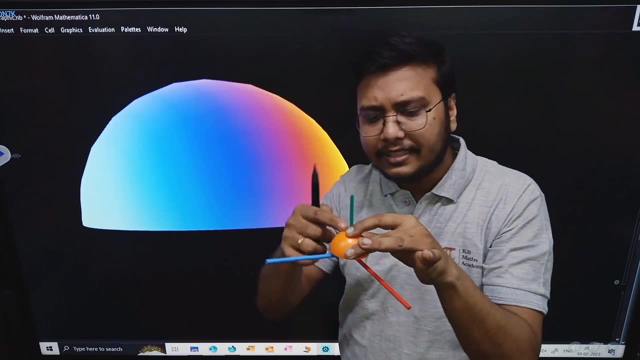 If this is the X axis, the Y axis, the Z axis, then a right-handed screw would advance in this direction. Now there is another way we can understand the direction of end cap, That is, if someone is walking around along the boundary of the C surface. 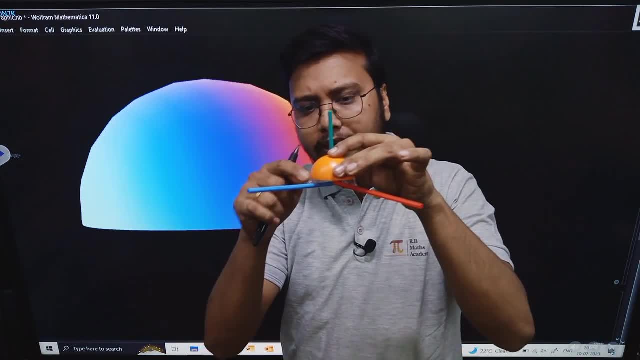 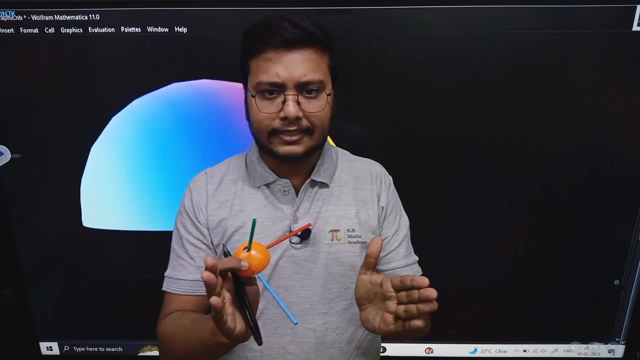 OK, imagine That someone is walking along the boundary, along this surface, in such a manner that the surface should be always on his left side. OK, so I'll be walking in such a way that the surface is always on my left side and the 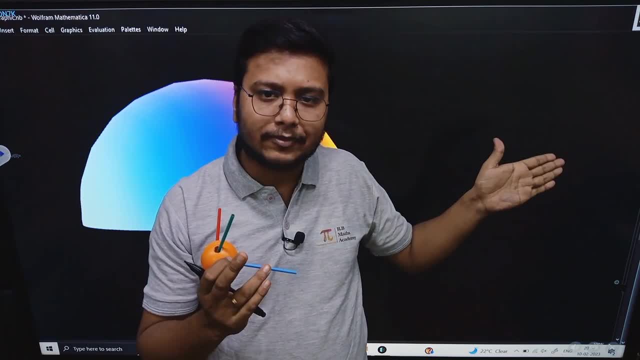 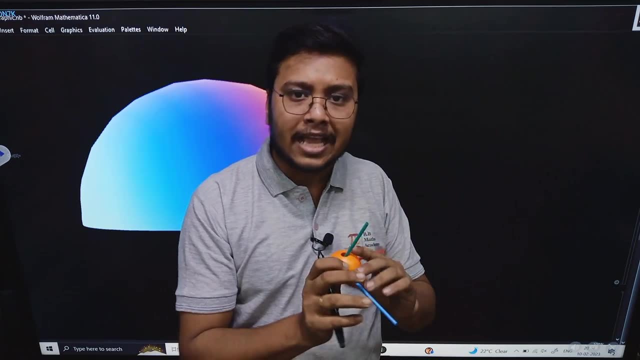 direction in which I need to walk by keeping the surface on my left, left side. that should be the direction of the C, the direction in which we are taking C. And now, if a screw moves in that particular sense, the way it would advance, that's the. 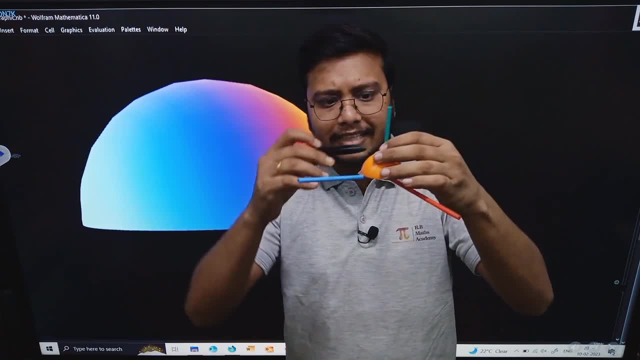 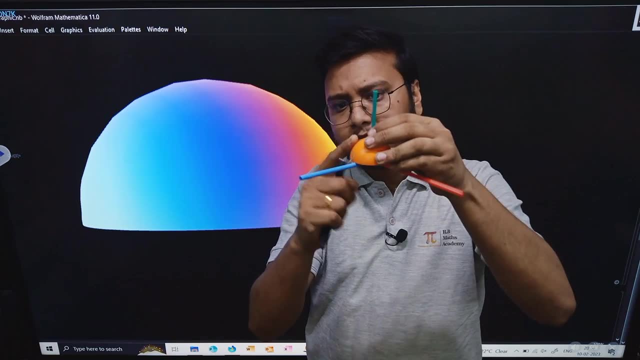 direction of end cap. So you can understand. in this particular case end cap is this direction, but not always like this. If I take a point on the S surface, the S surface on the S surface, if I take a point over here, then the end cap would be in this direction. 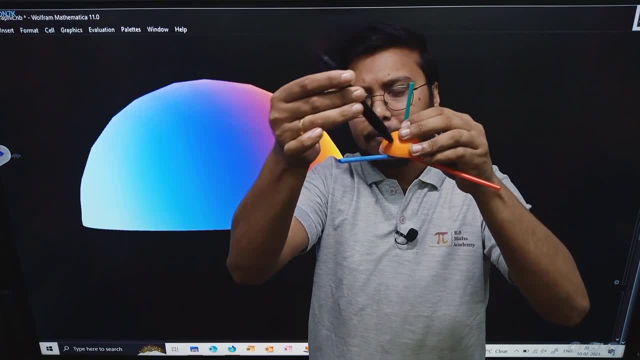 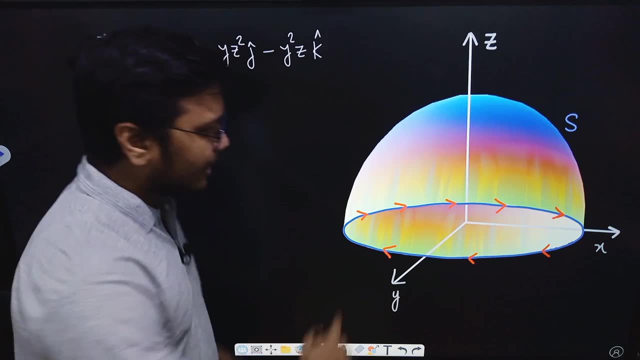 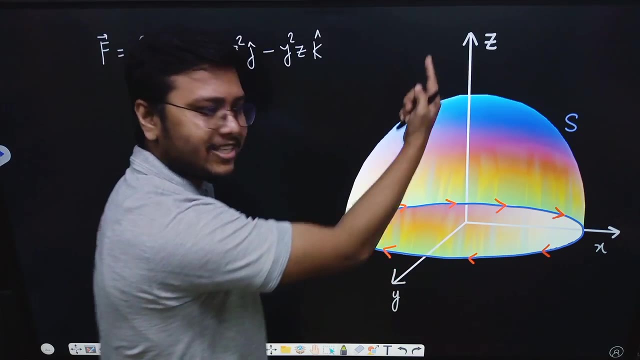 OK, something like this. OK, so the end cap direction is perpendicular to the surface and upwards, not downwards. OK, so, coming back to the problem, this is our hemisphere and we are moving in this particular sense. Then the screw is advancing in the direction of Z axis. that means upwards, but obviously. 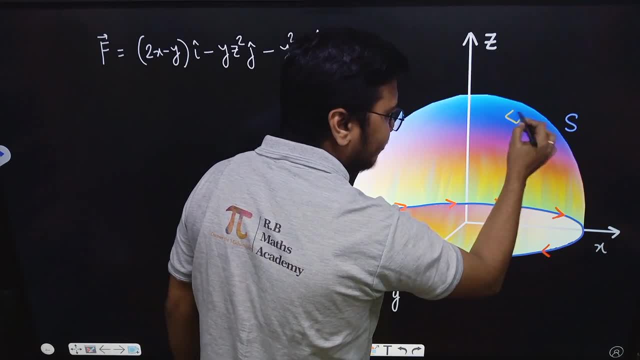 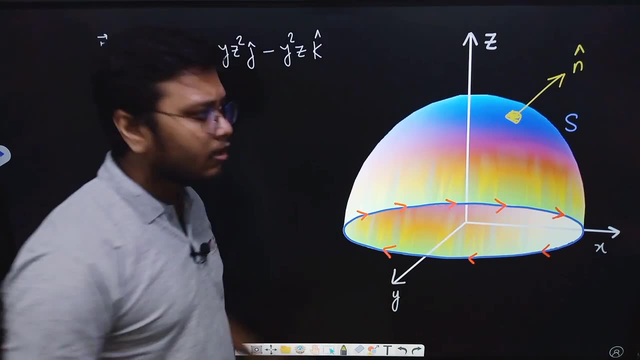 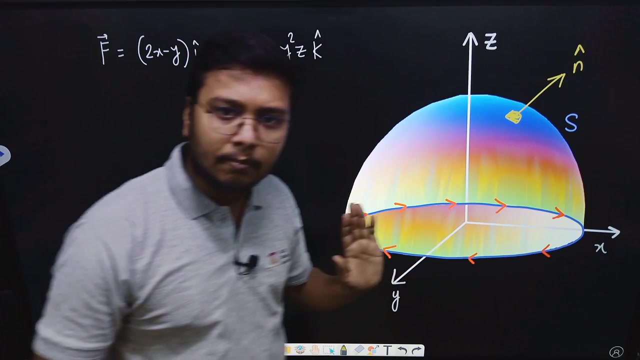 perpendicular to it. That means if I take any particular point on the surface S, then the end cap direction is something like that which is towards the direction of Z axis. that means upwards, but obviously perpendicular to the particular surface. OK, so we need to figure out what our end cap is. 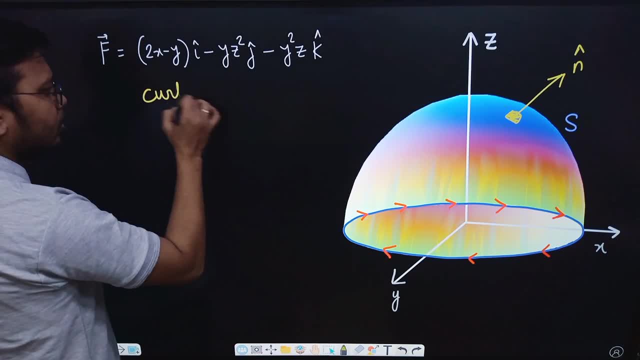 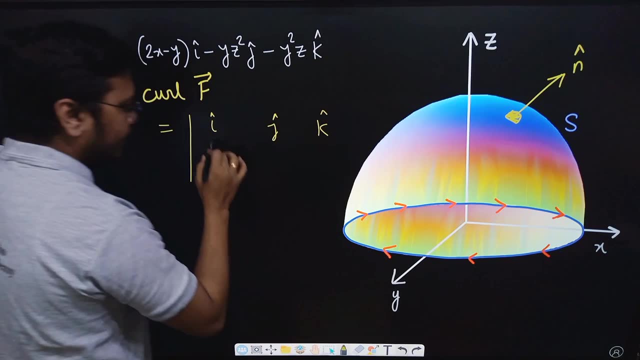 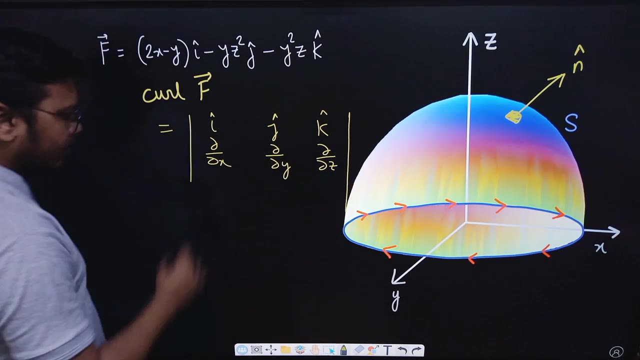 But before that let's Let's first find out curl of F. so curl would be determinant: i, cap j, cap k, cap del del x, del del y, del del z taken, and now we need to take the coefficients of the F vector. 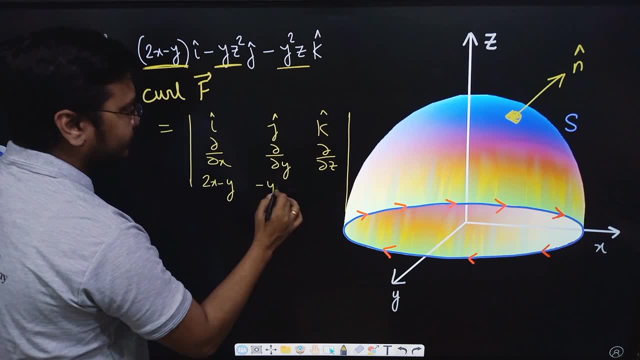 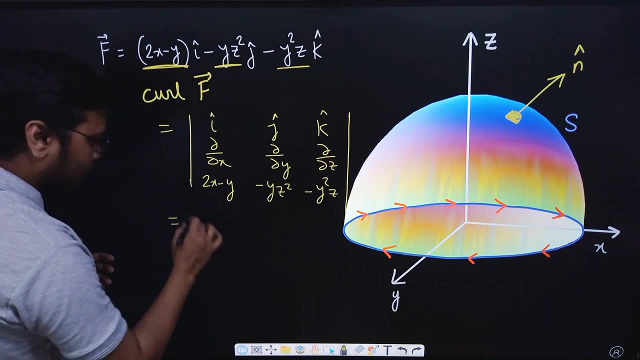 So that would be 2x minus y, minus y z square and minus y square z. So So if we just break up the determinant, so i cap when I'm breaking- I'm having a del del y of minus y square z and that would be minus 2y z, minus of del del z of minus y z. 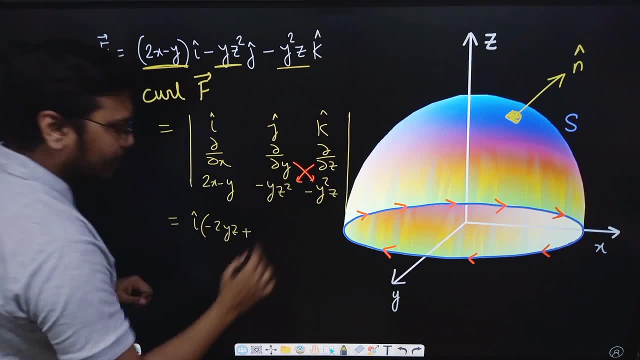 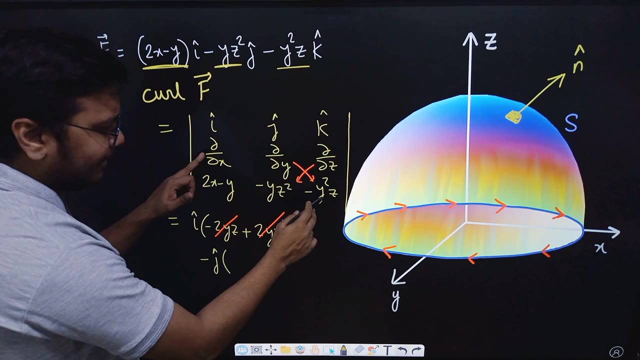 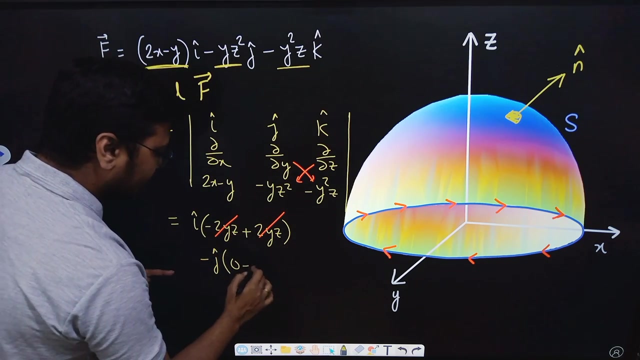 square. So that would be a plus of 2y z, right? So basically they'll just cancel up and become zero minus j cap. OK, so now If I expand along the j cap, then I'll be having del del x of this variable, that would be zero, and del del z of 2x minus y, that would be again zero. 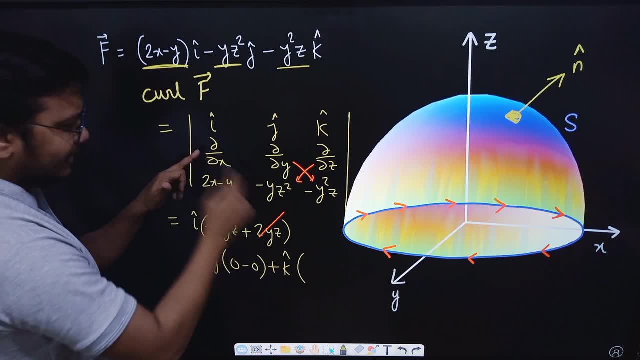 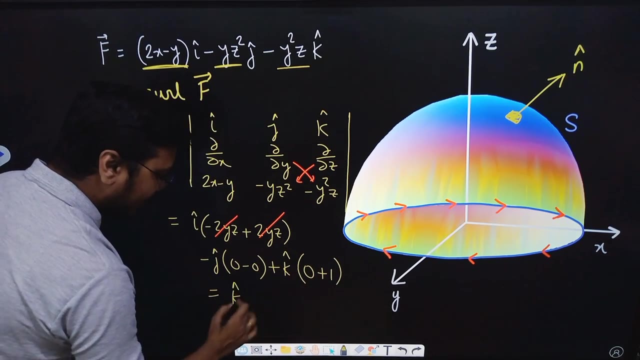 OK, so plus k cap of del del x of minus y- z square, that would be zero. and minus of del del y of 2x minus y, that would be again a minus one. So minus and minus, it will become plus. So we are simply having k cap as our. 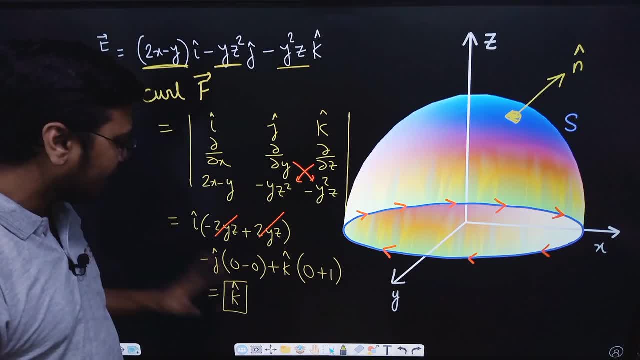 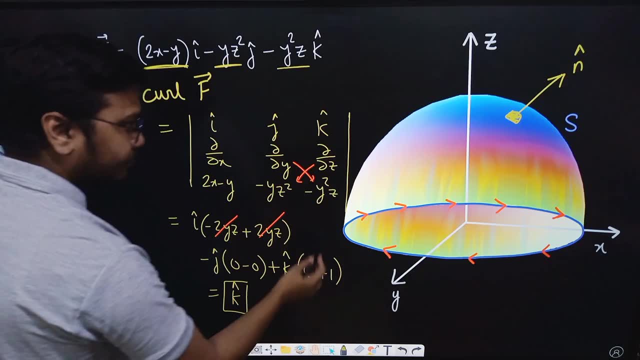 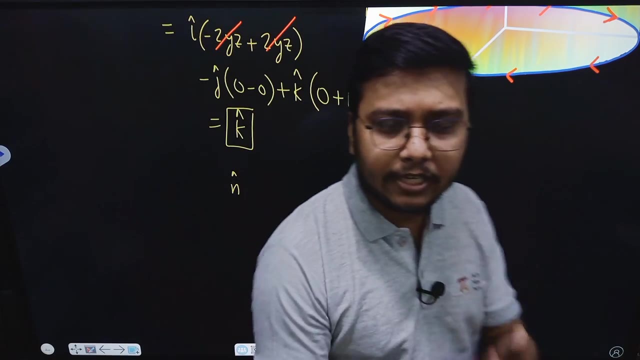 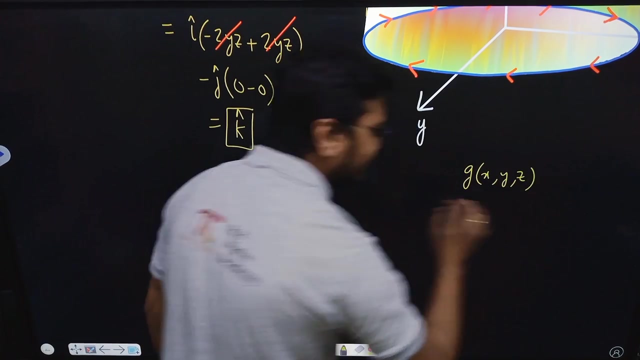 Curl of f. OK, so we have the curl of value and that's k cap. Now let's try to find out the in cap value. OK, So we already know that if we are trying to find out a unit normal perpendicular to a surface, then if the surface equation is given by, let's say, g is some function of x, y, z. 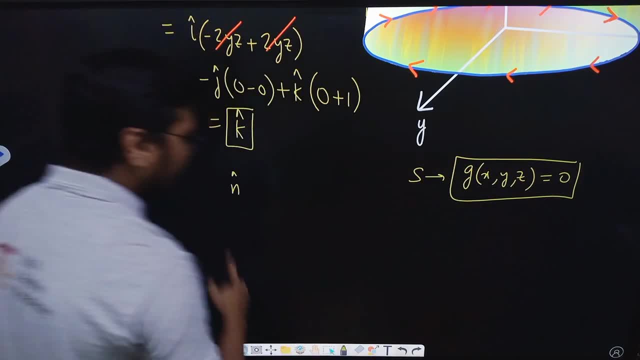 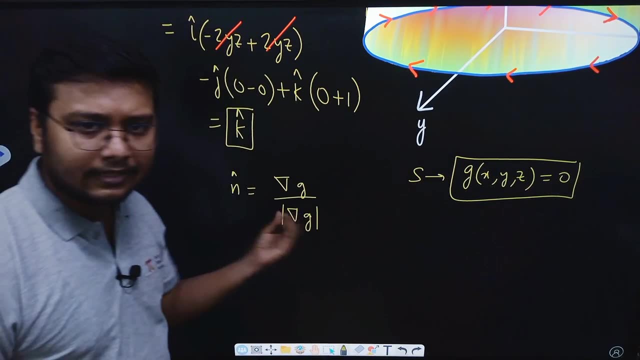 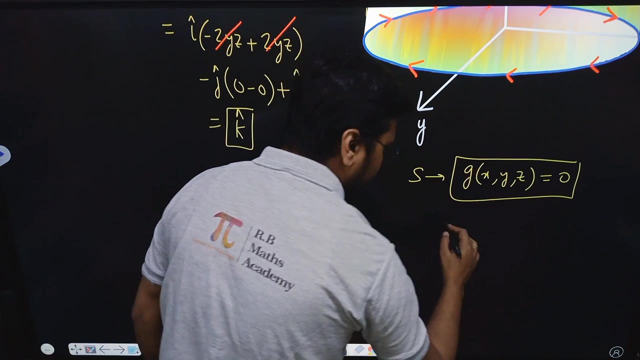 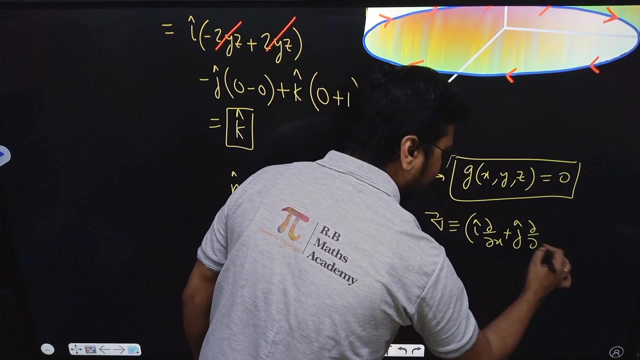 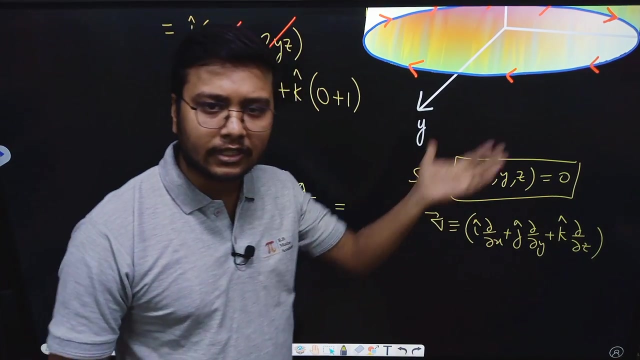 If this is the particular surface, then we know that In cap is grad g by modulus of grad g. right, That's the way it is done. So now grad of g would be. we know that grad function is nothing but i cap del del x plus j, cap del del y plus k, cap del del z and my g function, which is a surface. 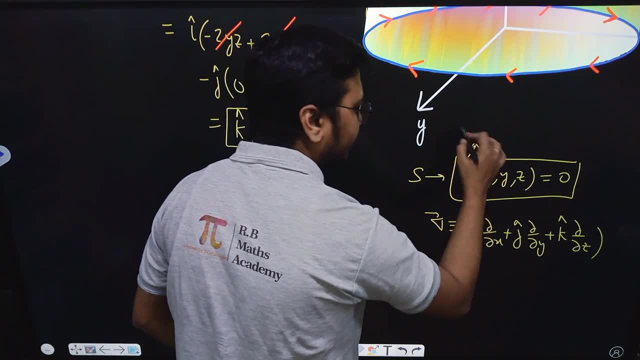 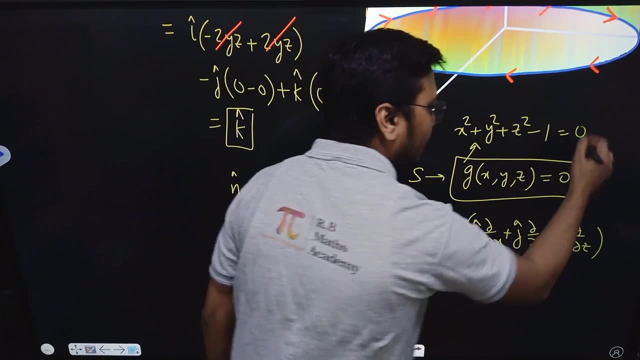 The equation of the Surface Of the hemisphere that's basically given by x squared plus y squared plus z squared, We have equals to one cell. bring the one on the left hand side, So it will be minus one equals zero. So that's the equation of the surface of the hemisphere. 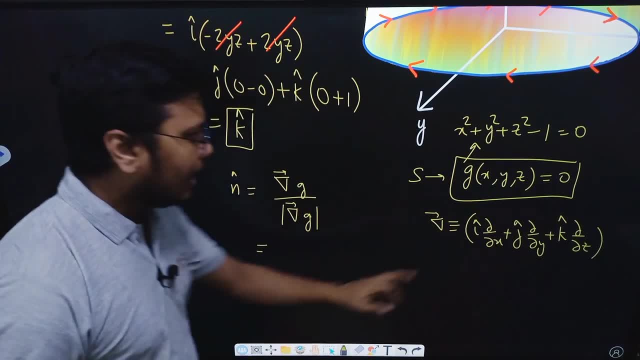 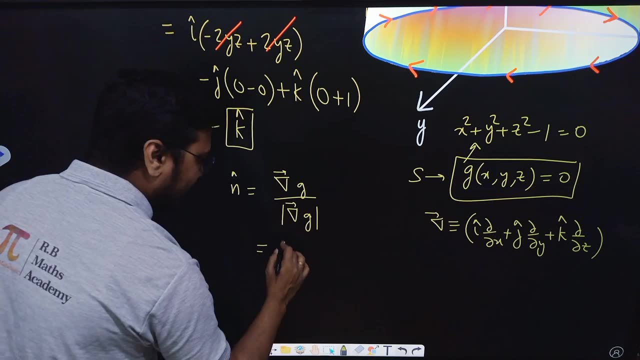 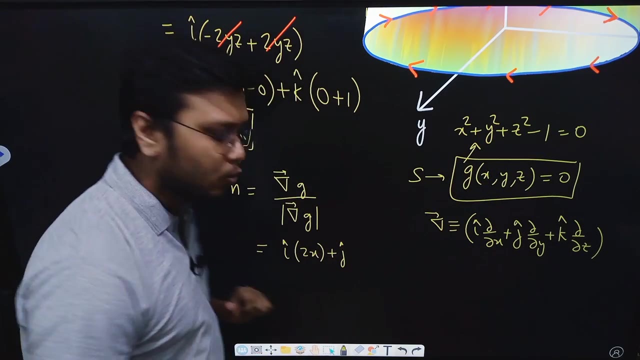 So grad of g, that would be Del del x of this value. del del x of this value is nothing but two x. So I'll be having i cap two x plus j cap del del y Of Again the same function, that would be a two y. 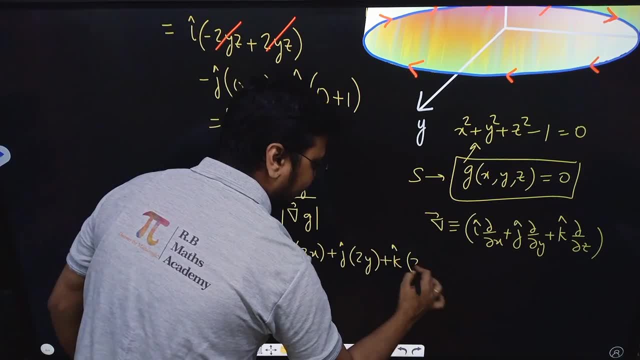 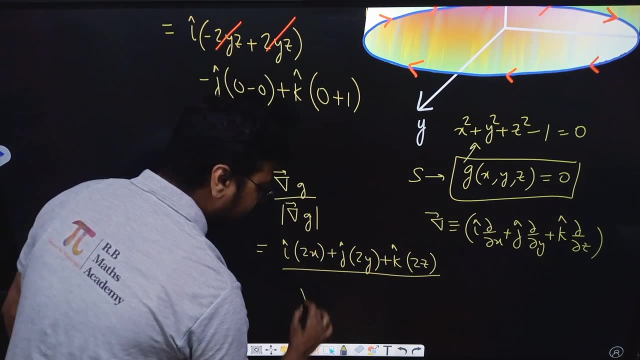 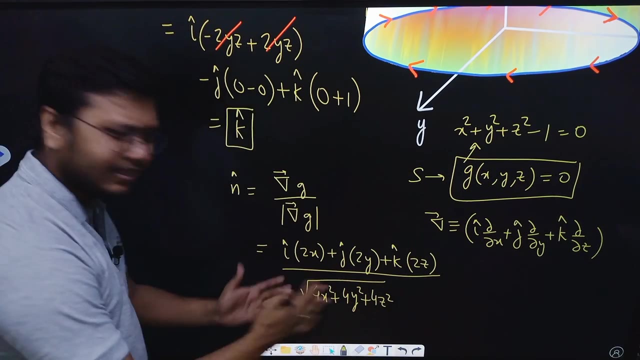 So two y and similarly k cap of two z Right divided by modulus of this vector, quantity. modulus of this vector would be root over of four x square plus four y square plus four z square. So you can just visibly see that the two and the force inside the root over will simply cancel out. 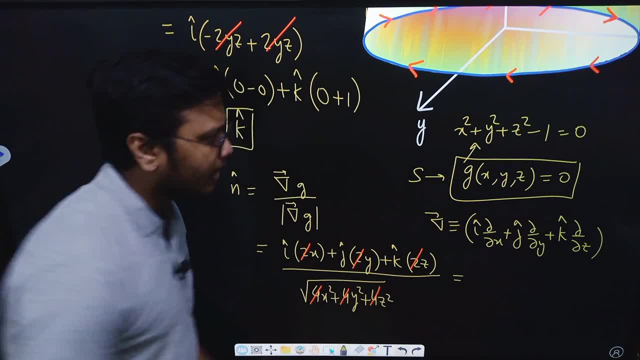 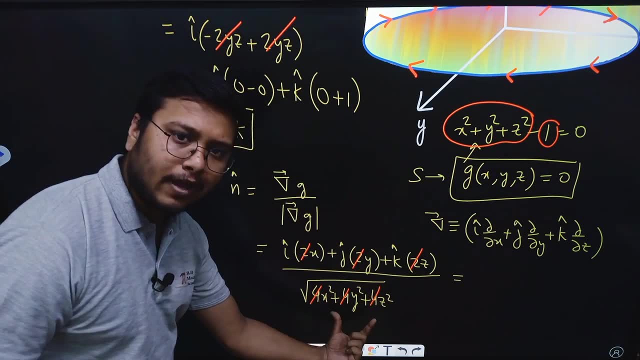 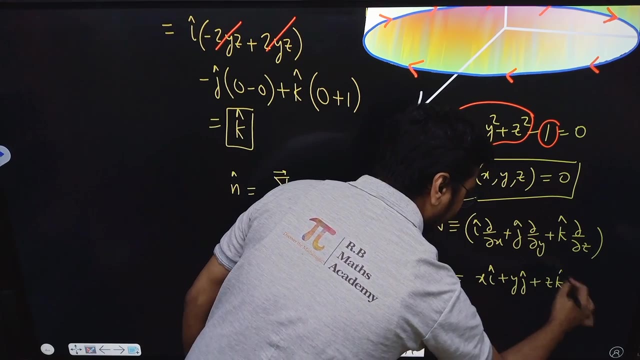 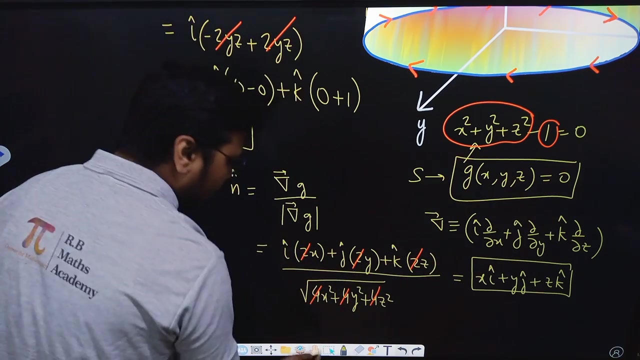 And here in the denominator I have x squared plus y squared Plus z square, and I know that the value of x squared plus y squared plus z squared is nothing but one if I take the one on the right hand side. so the denominator value is becoming one. so all I have is x i cap, y j cap plus z k cap. okay, so that's my unit normal vector. okay, now we know that using stokes theorem, 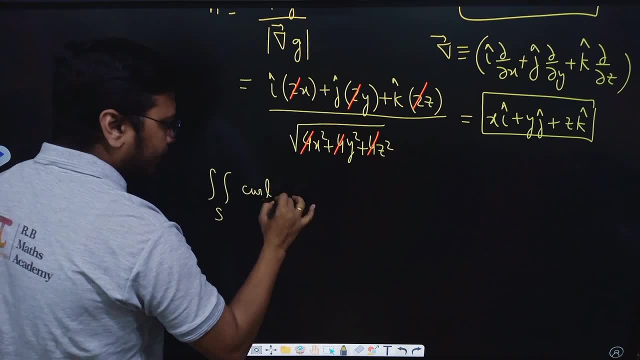 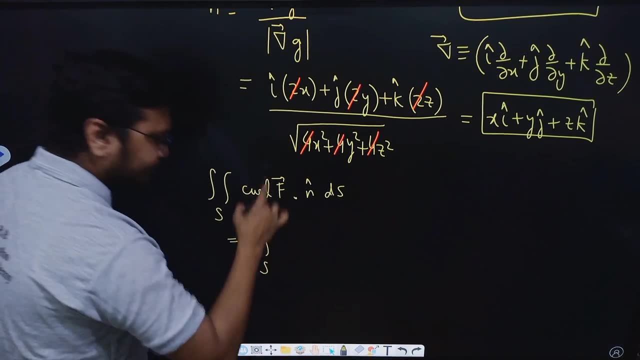 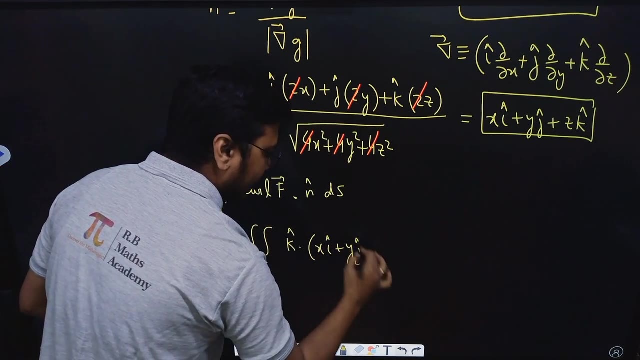 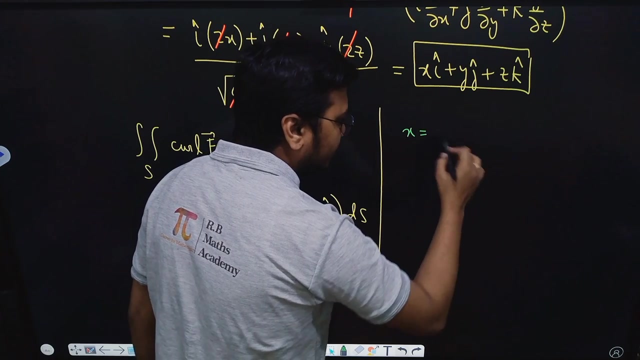 We need to find out this value, Curl f dot in cap ds. And we have got the values to be: Curl f value is k cap dot in cap value is x, i, y, j and z k cap ds. So it is better to take a substitution: x equals r cos theta and y equals r sine theta. 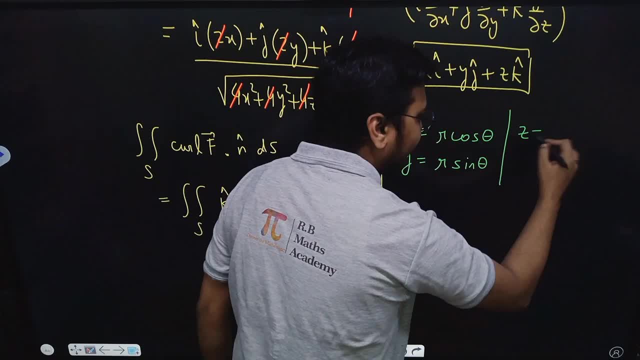 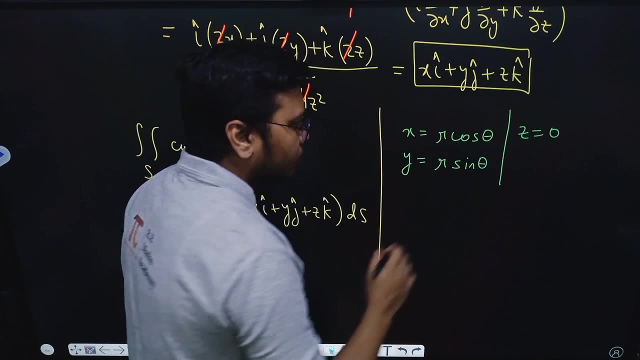 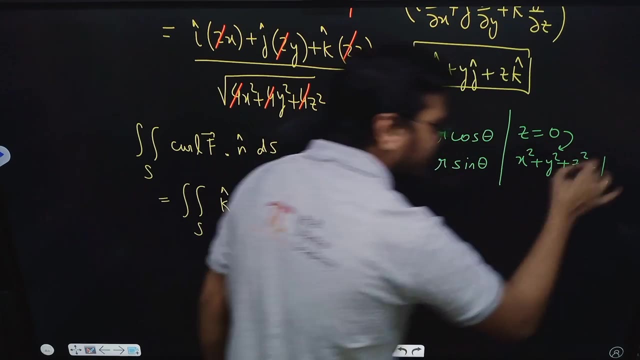 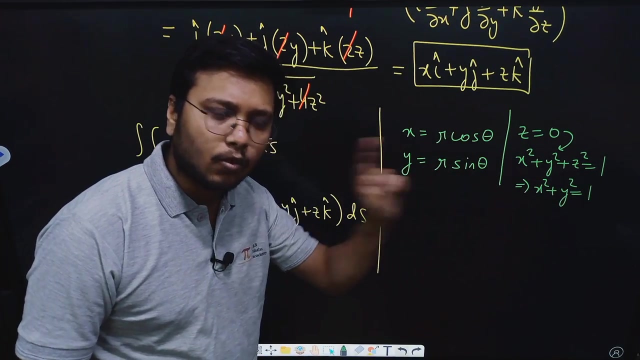 Now, in this case, when z equals to Zero, okay, when z equals to zero, that means along the c boundary. on along the c boundary, the z value is zero. So z value is zero and in that case the value of x squared plus y squared plus z squared equals to one. if I substitute z equals to zero, it becomes x squared plus y squared equals to one, and that's a circle having radius one. 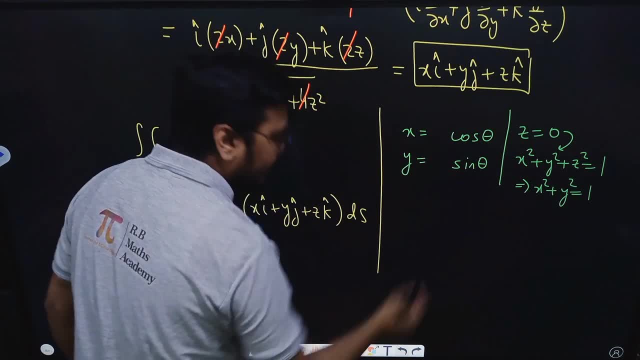 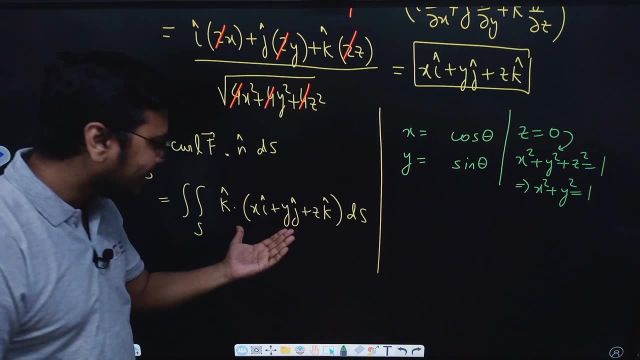 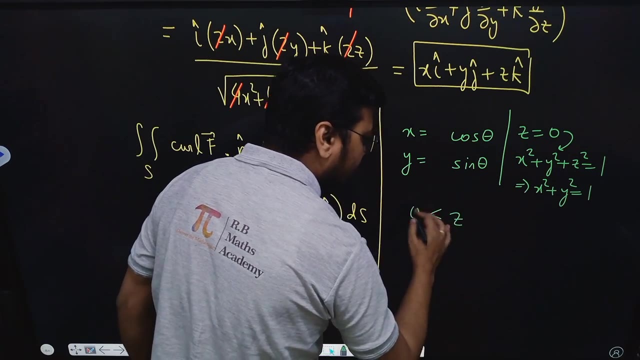 So in place of r I'm going to take simply one, So no need to write. so I'm having The substitution: x equals to cos theta and y equals to sine theta. I'm going to make that substitution here. And The z value that's simply going to range from zero to the total height of the hemisphere, which is nothing but one. 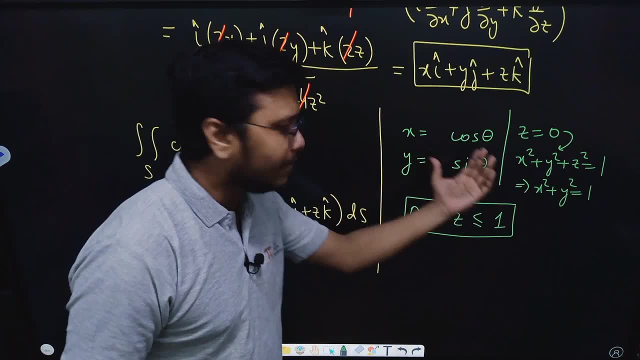 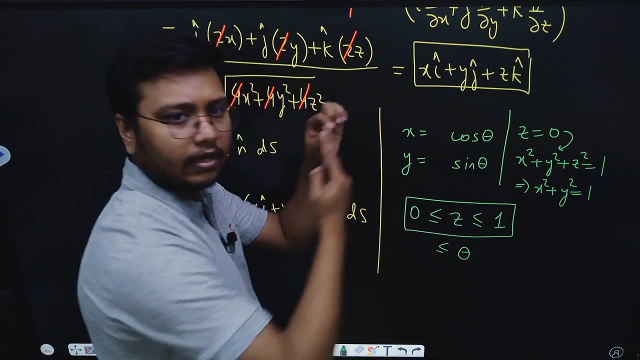 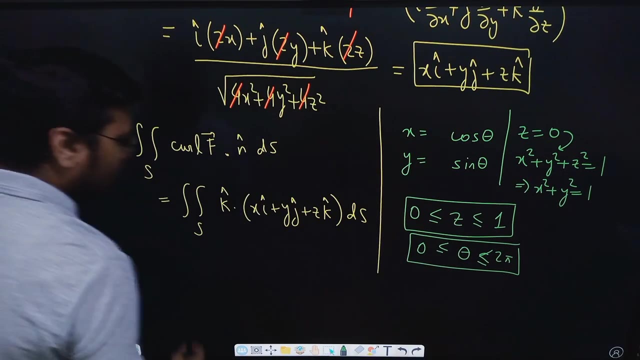 So z is going to range from zero to one, and x and y- I'm taking this substitution- where obviously the theta is going to range from- since it's a hemisphere, a total round figure- so from zero to two pi. Okay, So I'll come back to the problem. 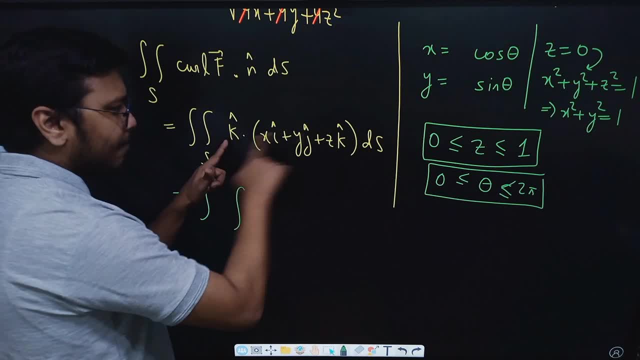 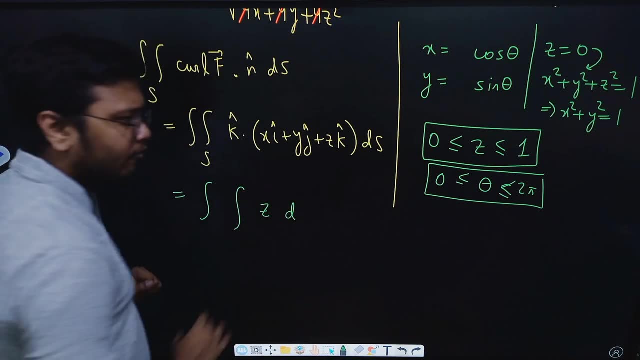 Now, if I try to make these substitutions, K cap, dot k cap, that will be one. so all I will be having is said: and in place of d x, I want to write d Theta and d z, because those are my variables now. And 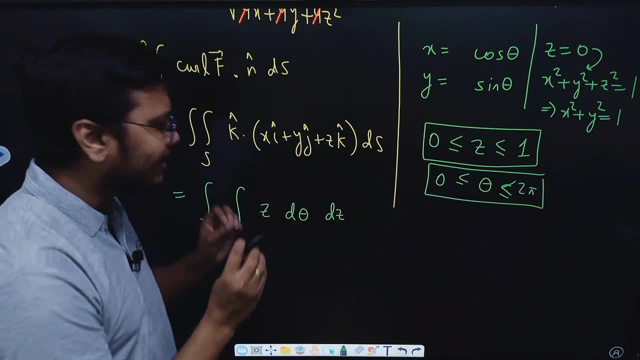 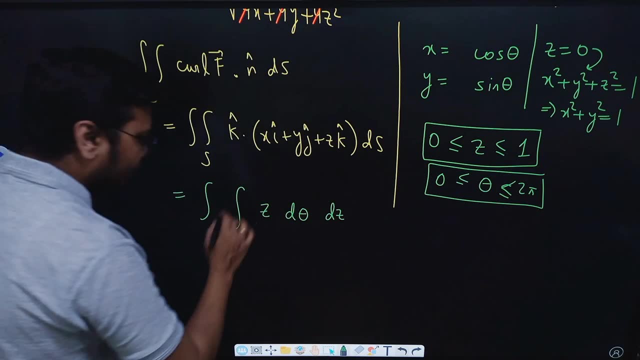 Obviously, when I'm making a substitution, I Need to think about the Limits. Okay, right, how the limits are going to change. So Here you can understand that the z limit is going to vary from, as you can see, zero to one. So the z limit is going to vary from zero to one. 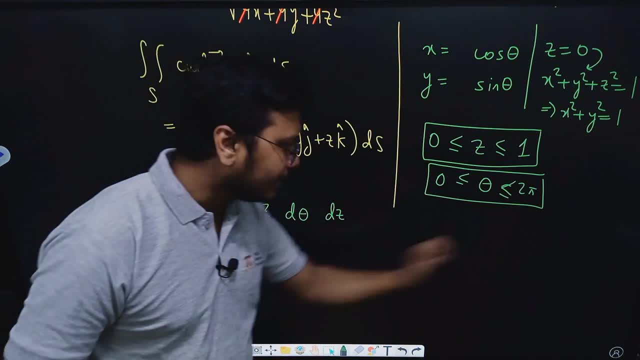 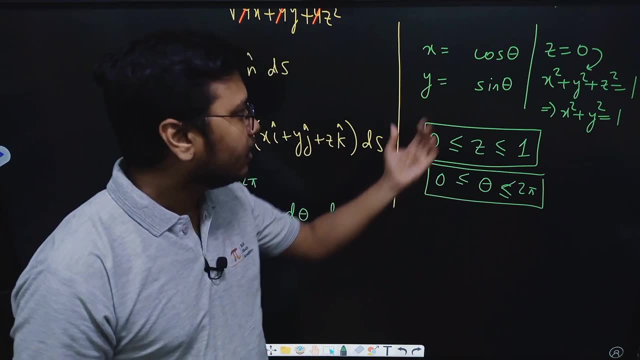 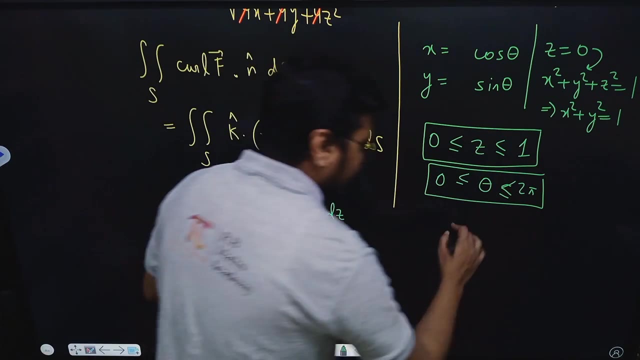 And The theta limit is going to vary from Zero to two pi And in a multiple integral. Whenever We take a substitution, you need to keep in mind the Jacobian Right. The Jacobian is going to be The Jacobian value. 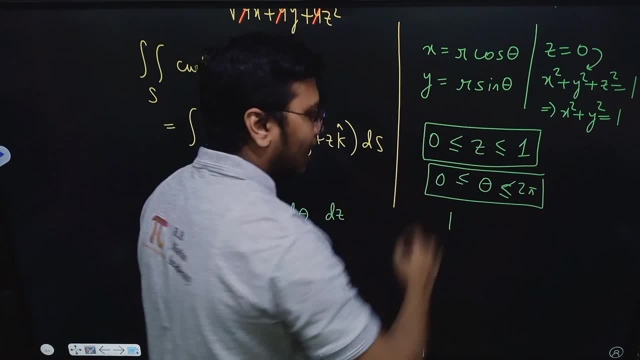 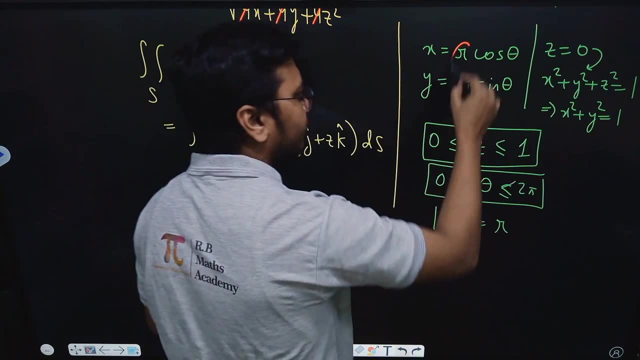 The Jacobian value. if we take x equals to r cos theta and x equals to r sine theta, Then the Jacobian, or the mod Jacobian value is nothing but r, And in this case we have taken r to be equals to one. So that means my Jacobian value is also one. 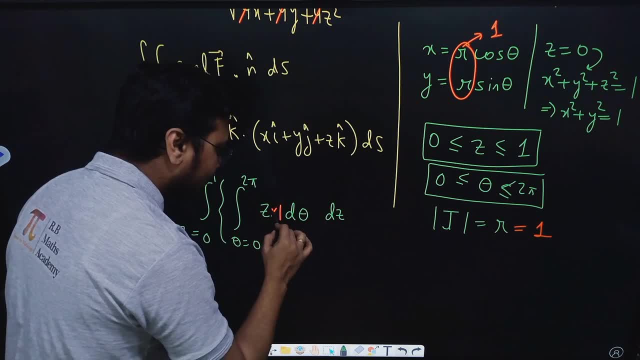 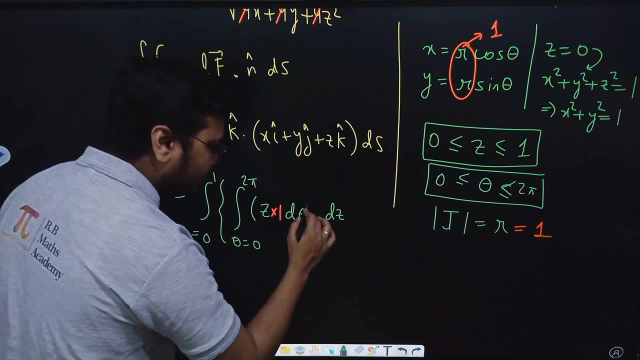 So I just need to multiply a one, which is the Jacobian value, Since I'm making a substitution in a multiple integral, So it doesn't make any change over here in this case. So first of all I'll do the integration with respect to theta. 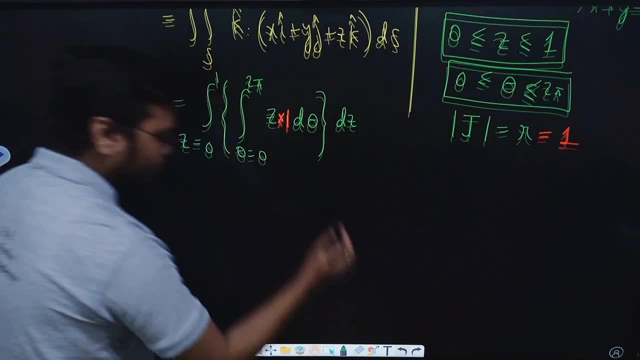 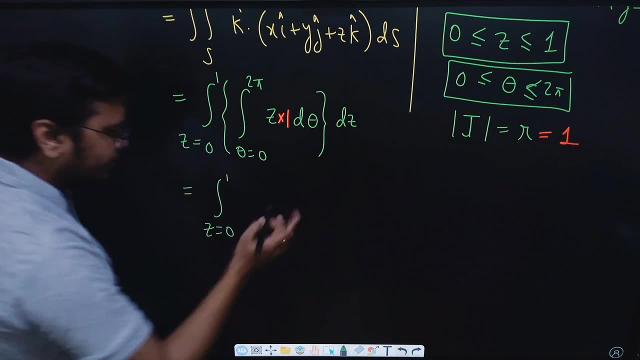 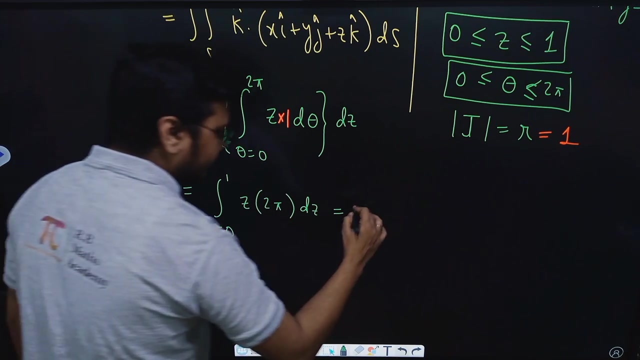 And then, with respect to z, Z equals zero to one. Z is not dependent on theta, So I'll simply have z times the upper limit, which is two pi dz And Two pi z, square by two Zero to one, And that's going to be. 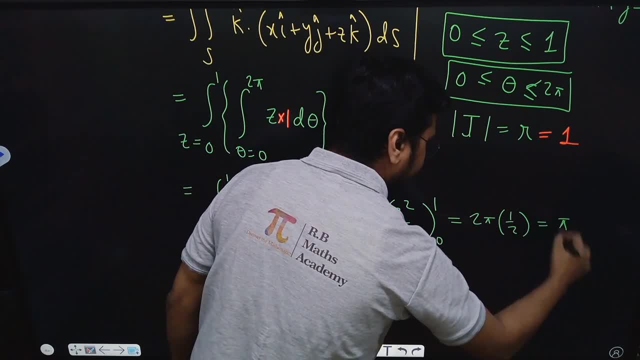 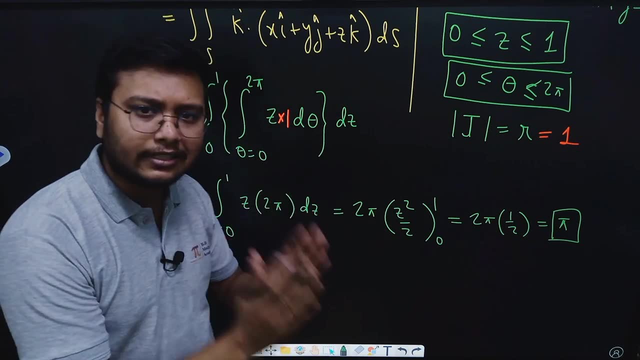 Two pi times half And that's just simply pi. So that's the value using the right hand side or the double integration in the Stokes theorem. Now we need to verify Stokes theorem here, So we need to do the left hand side also. 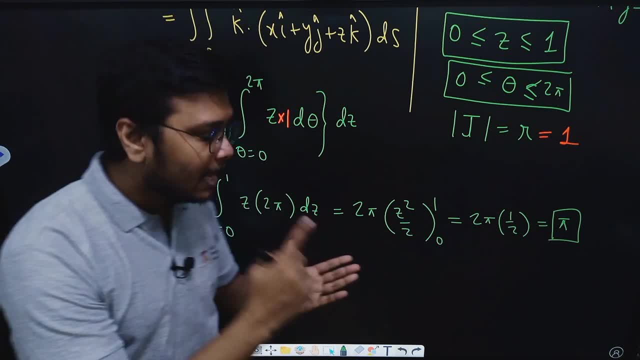 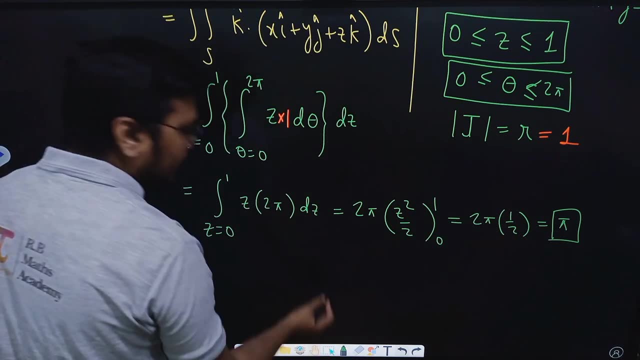 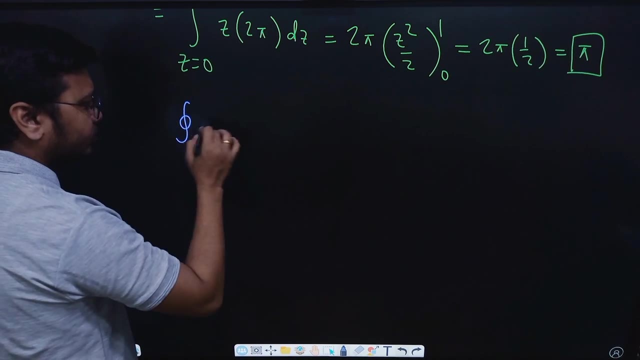 Where we will have to do the integration along the curve C, The closed integral along the curve C, And try to get the same answer, which is pi. Okay, So Let's now start with The other part of Stokes theorem, Which is the closed integral. 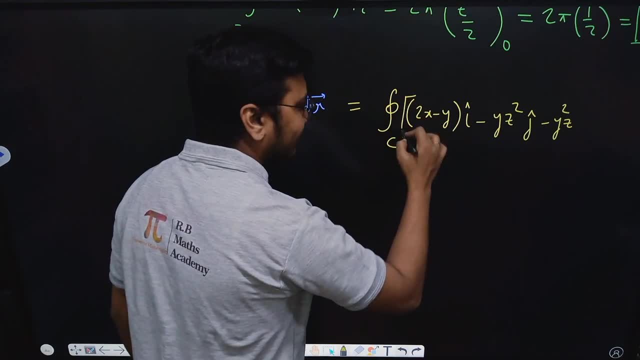 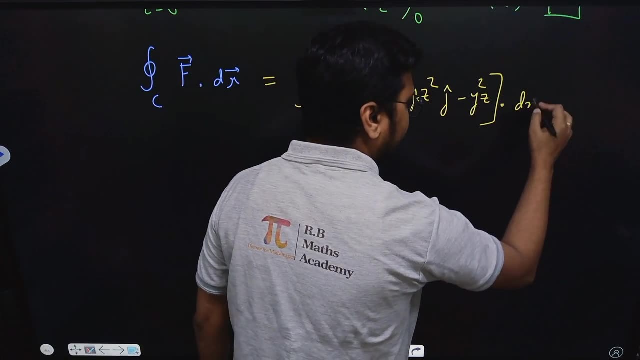 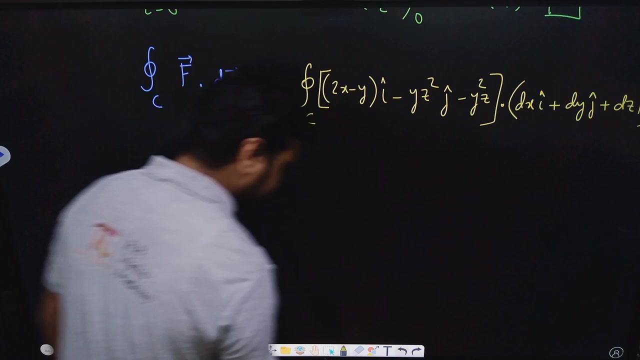 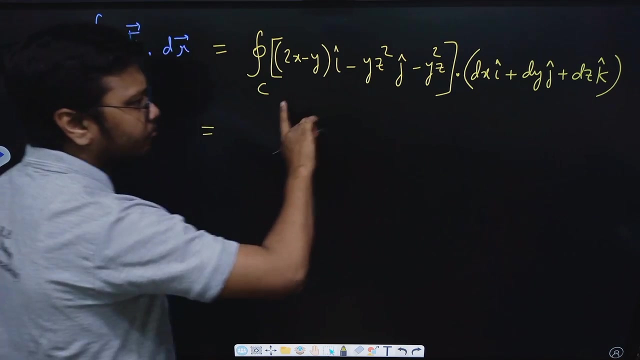 F dot dr. So that's the F vector Dot dr. Now I'm taking dr as dx i cap plus dy j cap plus dz k cap. Okay, So that's My Closed integration. So if I just Do the 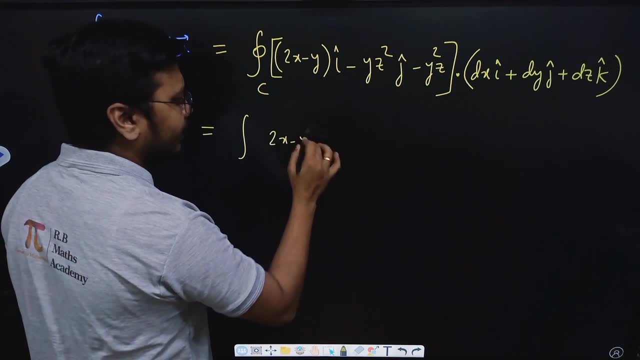 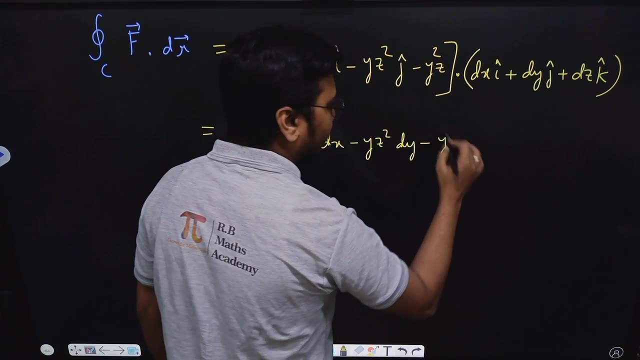 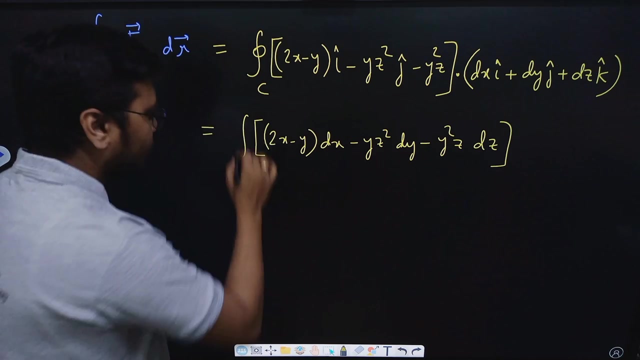 Corresponding multiplications, Then I'll be having two x minus y dx And Minus y z square dy, Minus y square z of dz. So that's the integration I need to do along the curve C. So Now, 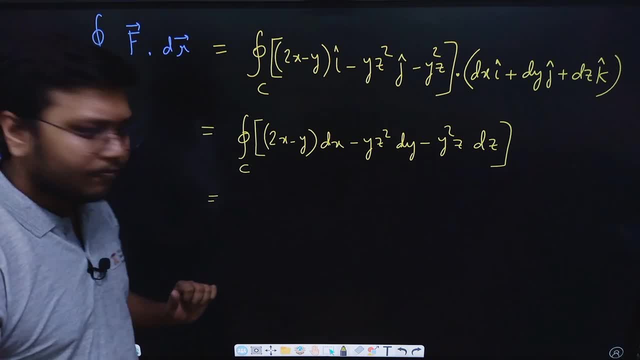 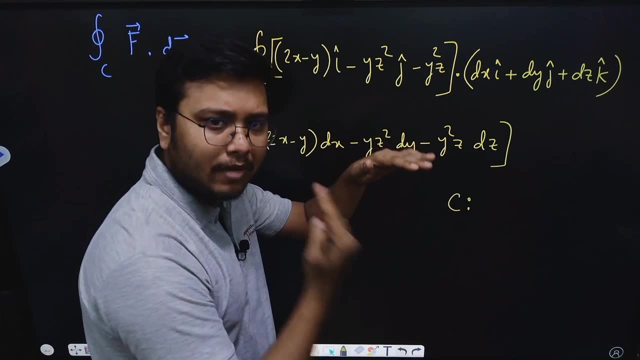 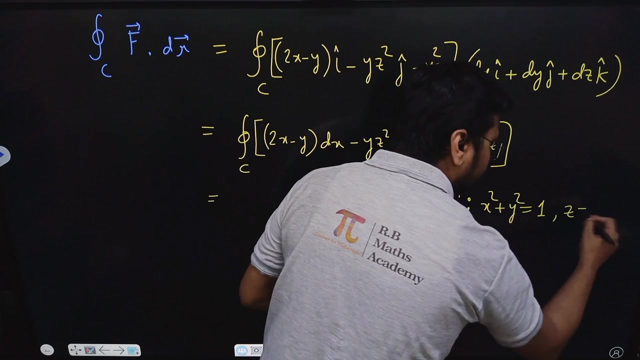 How do we proceed with this kind of integration Along the curve C? We know that the equation of C? C is nothing but a circular base of the hemisphere. That means x square plus y square equals 1.. And the value of z is particularly 0.. 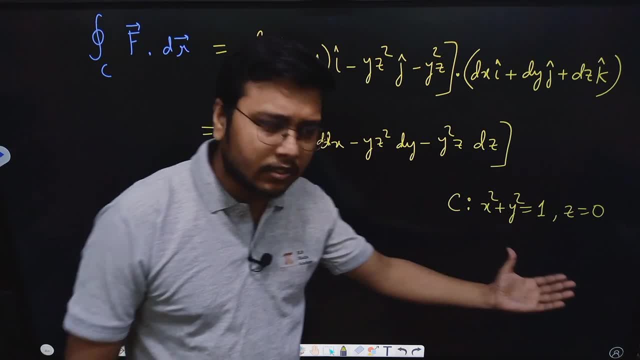 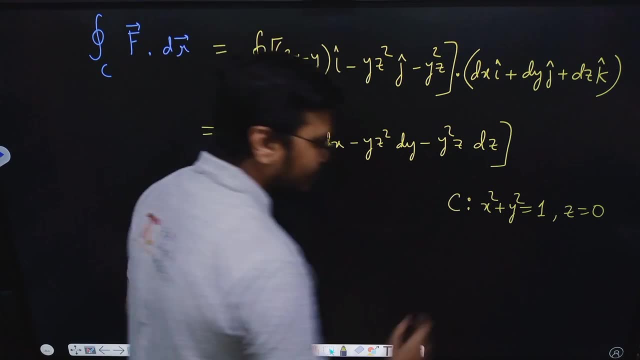 So we can again make a trigonometric substitution here, Or we can Do any way that We are comfortable with. So I'll just Make the substitution. That would make the problem easy. So obviously I'll take x equals 2 cos 3.. 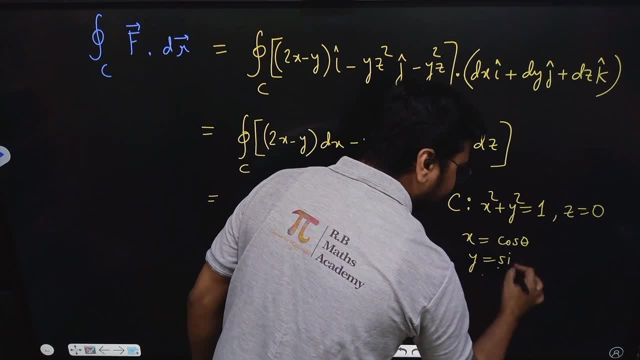 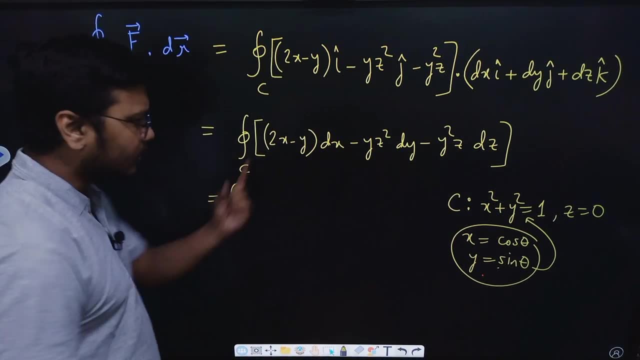 And y equals 2 cos theta And y equals 2 sin theta. So this would Definitely satisfy that circle. So If I take, If I put x as cos theta, Then it's going to be 2 cos theta Minus y. 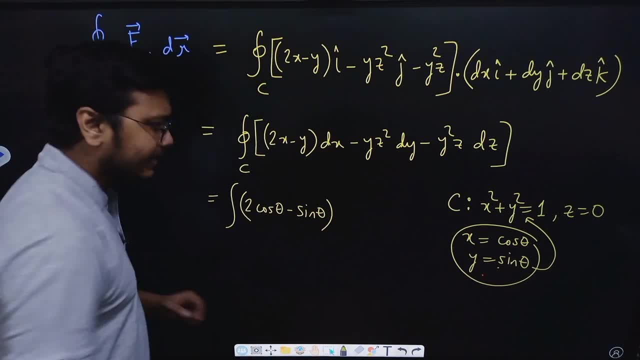 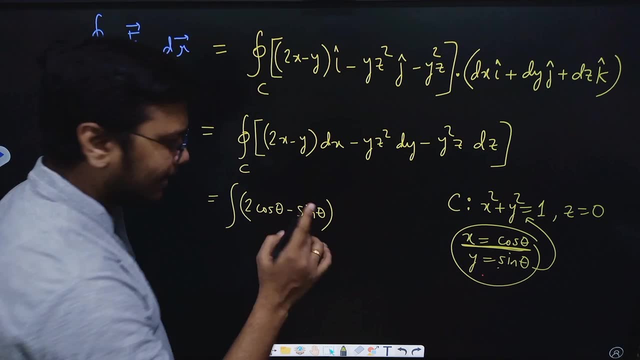 That's going to be sin theta And dx From this line, Obviously you can understand, the dx value is going to be Minus sin theta, times d theta. So minus sin theta, theta d theta Right. So that's the. 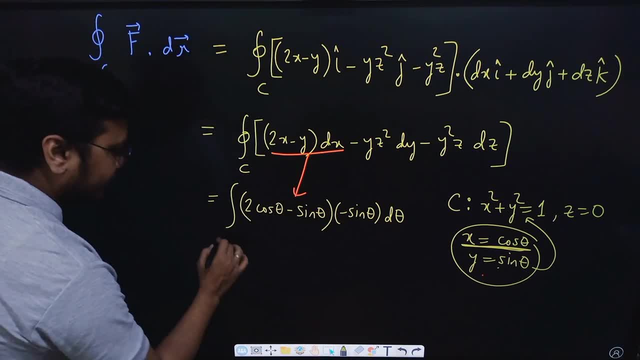 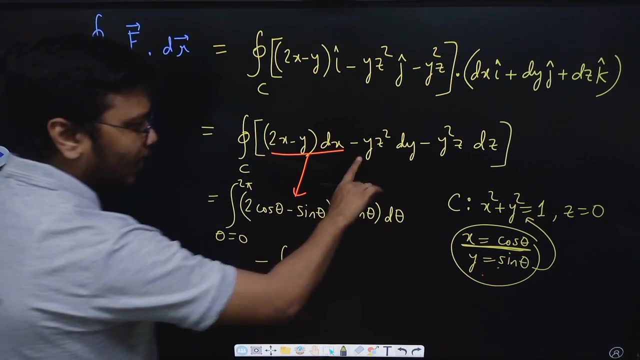 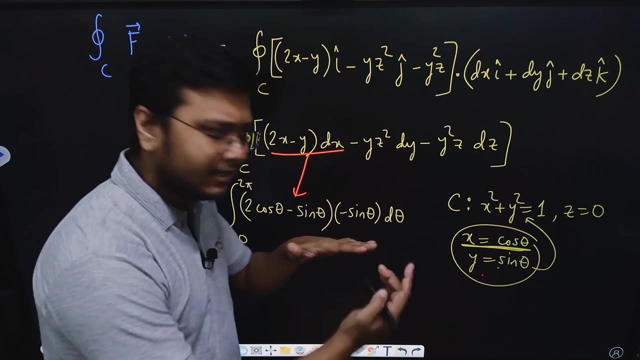 First Part We have got And obviously theta is going to vary from 0 to 2 pi Minus. Coming to the second part, y z square Right. So Value of z is definitely 0.. Along Where the c. 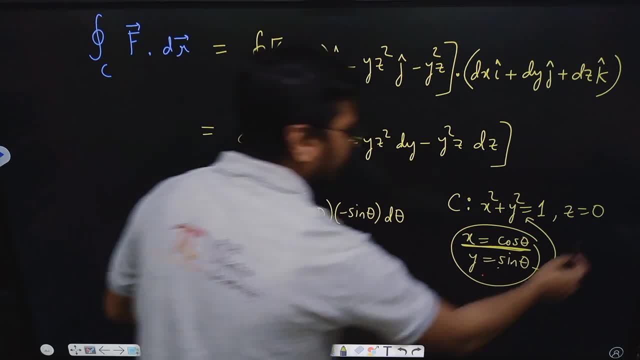 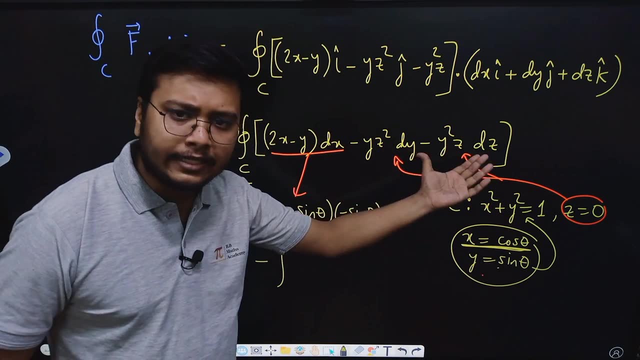 Curve is lying. The value of z is 0. So if I just put the value, z equals 0.. Over here And over here, So you can understand the Two, The second and the third integrations: They are becoming 0.. 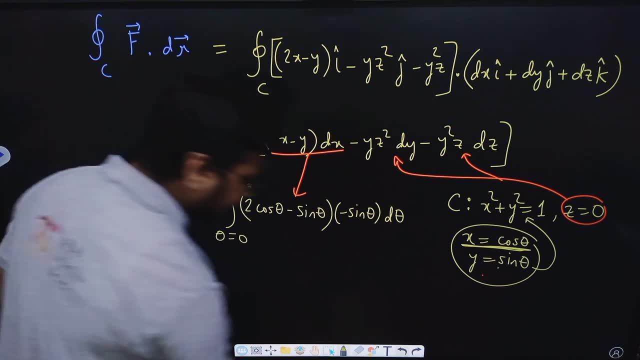 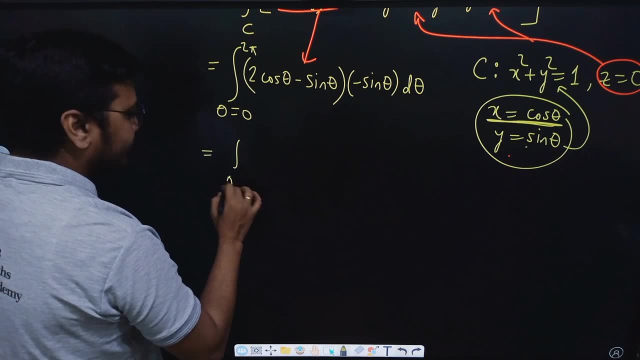 So I just don't need to Write them anymore. Okay, So if I now proceed with this particular calculation, If I multiply It's going to be theta from 0 to 2 pi. I'll have 2 cos theta times sin, minus of sin theta. 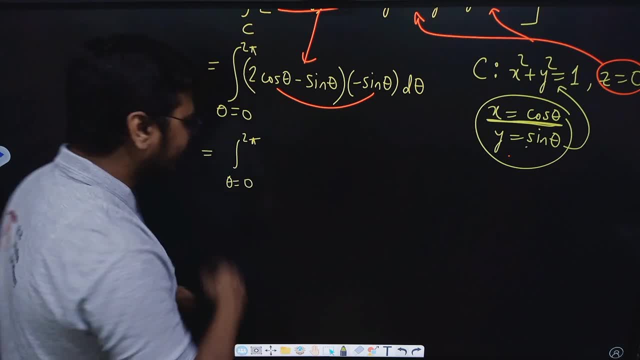 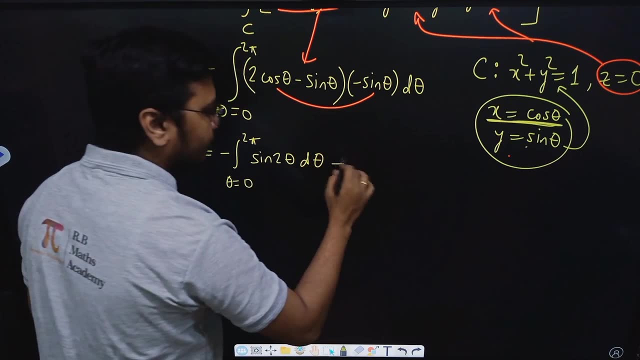 That's going to be 2 sin theta. cos theta, That's sin 2 theta. So minus common outside Sin 2 theta. That's our first integration, And Minus minus It will become a plus Theta from 0 to 2 pi. 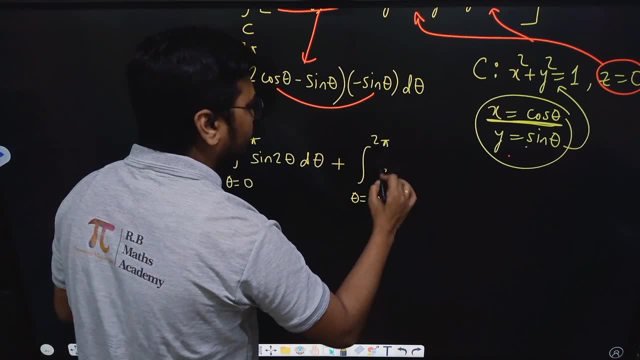 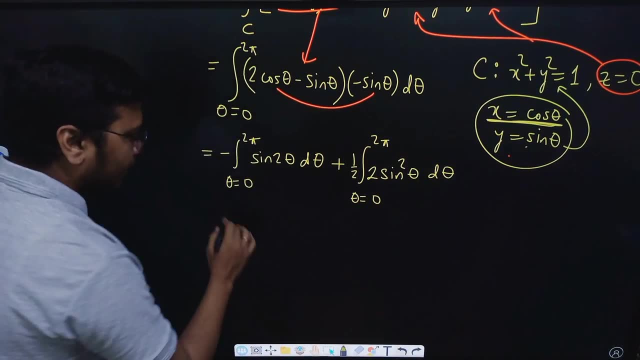 Sin square theta d theta. So we can adjust the second integration With a half outside And a 2 inside. So This first integration is going to be: The minus is going to become plus Cos 2 theta By 2.. 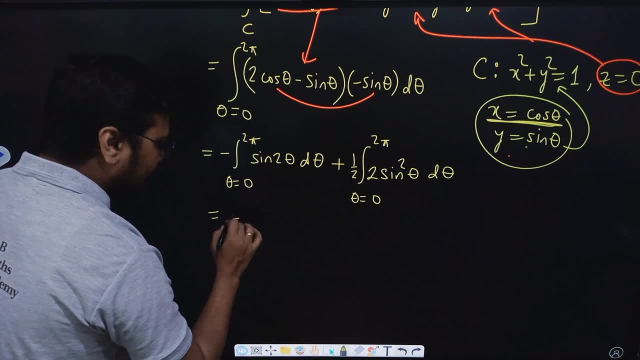 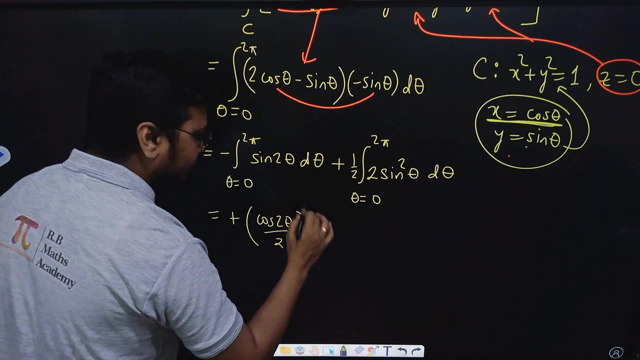 And Theta from 0 to 2 pi. And in the second case, 2 sin square theta Minus Theta Cos 2 theta By 2.. And Theta from 0 to 2 pi. And. 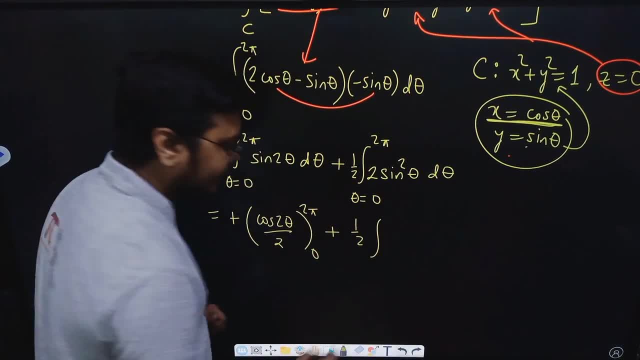 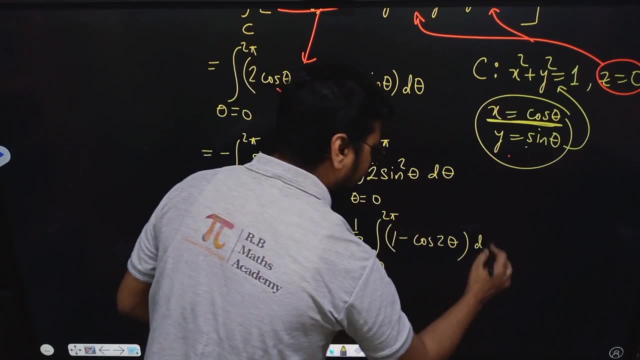 In the second case, 2 sin square theta Minus Cos 2 theta 0 to 2 pi d theta. So if I Put the limits in the first part, Cos Of 4 pi Cos. 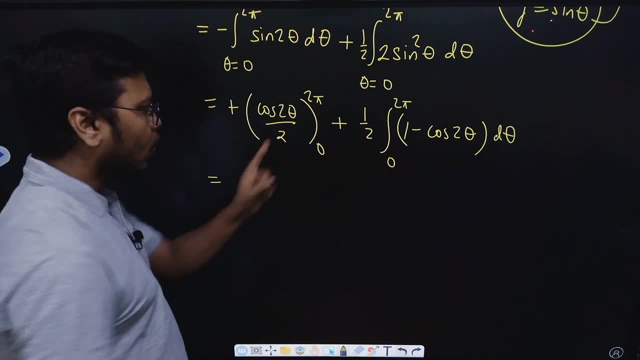 Of 4 pi, That's going to be Simply 1.. So I'll be having Half Minus Cos 0. That's again 1.. So minus Another half And That's becoming completely 0.. 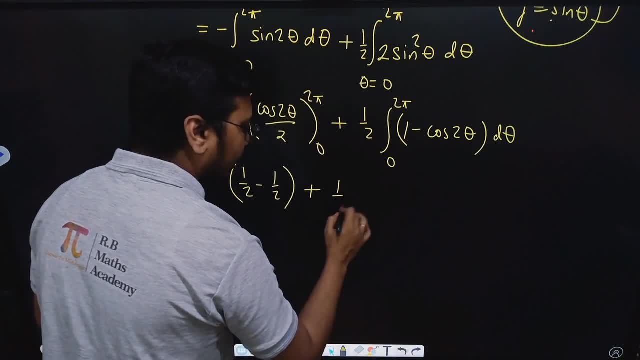 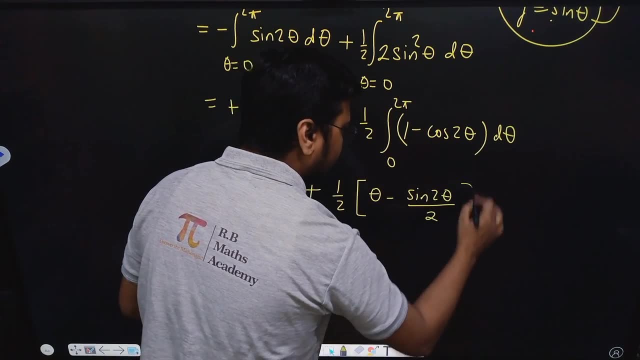 Plus Half. Theta Minus Sin 2. Theta By 2. Theta From 0 to 2 pi, So half. If I put 2 pi In place of theta, That's going to be a 2 pi. 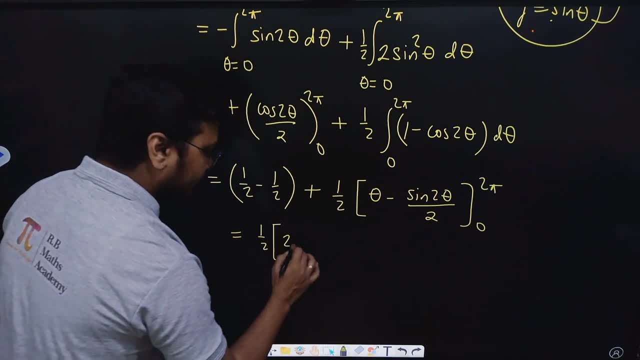 Minus In place of theta. If I put 2 pi, So sin 4 pi, That's going to be 0.. So minus 0.. That's the upper limit Minus. If I put the lower limit, Then both the values are going to be 0.